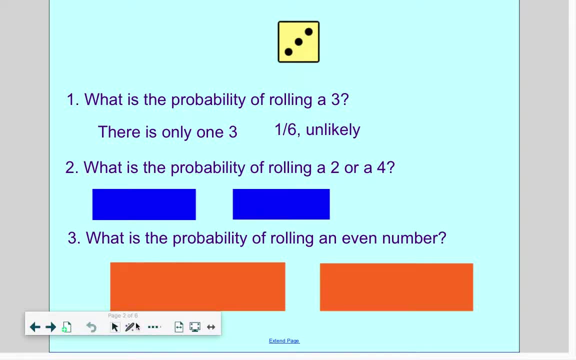 a two or a four. Well, I want to drag your attention right up here to this word, there, Or When we're doing probability, or really means, and So this question number two: what is the probability of rolling a two and a four? 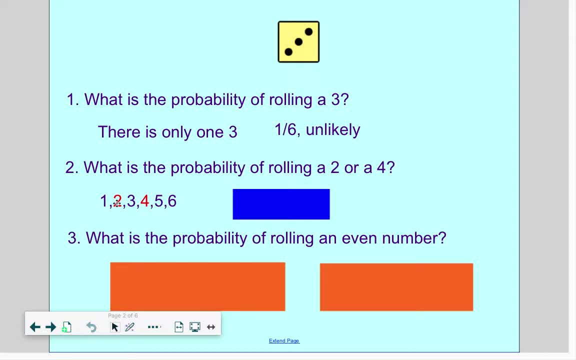 So if we were to look at all the numbers on this die, we have a one two and one four. So there are two numbers. we want it laying on Two out of six or a two six chance. Two again is not very close to six, so the word we would use for that would be unlikely. 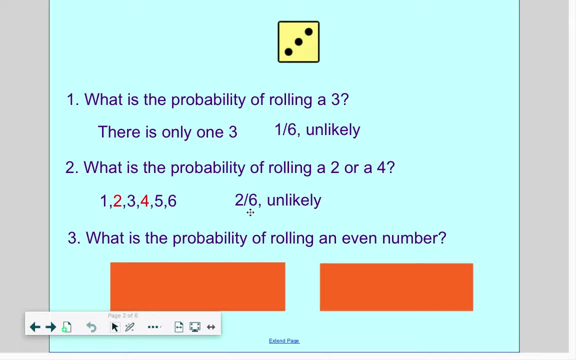 So a two, six. chance of rolling a two or a four, and our word would be unlikely. What's the probability of rolling an even number? So we roll this die up here. Our even numbers are two, four, six. Our odd numbers on this die are one, three and five. 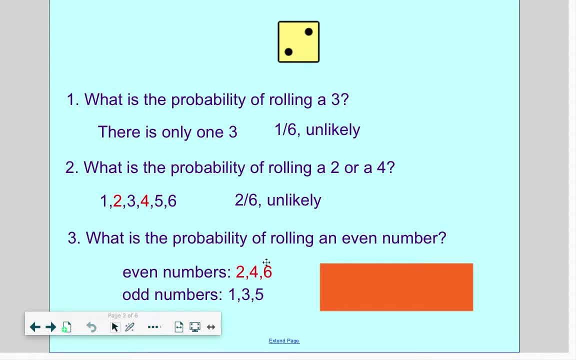 So they're asking about even. There are three evens, but there are six numbers total, So three sixths chance, Three out of six. Now, what I do want you to notice is: there are three evens, but there are also three odds. 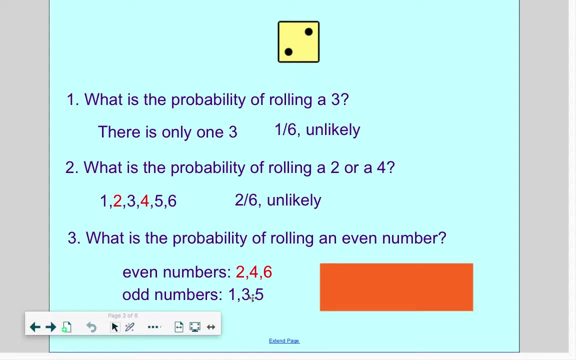 This number is equal To the odd number. Even numbers are equal to the odd numbers: One, two, three. One two, three. So therefore we have a three, sixths chance of landing on even numbers, and it's equally likely because we have the same amount of odd numbers on this die. 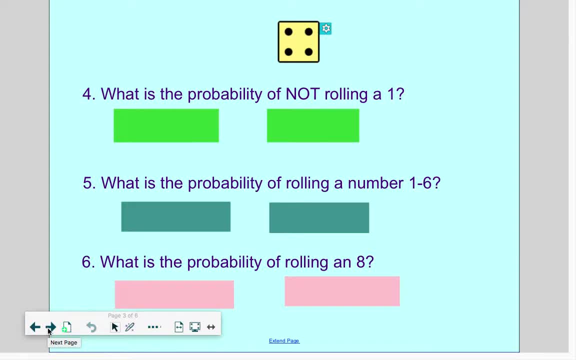 Alright. question four: What is the probability of not rolling a one? Well, when you think about all the numbers on a die there, they are right there. So the numbers that are not ones are two, three, four, five and six. 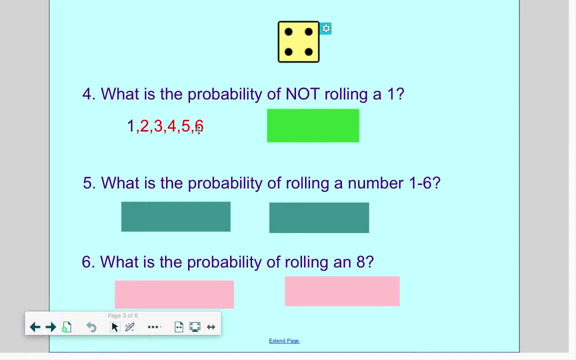 So that means one, two, three, four, five of my numbers are not a one, So five out of the six numbers on this die right here are not ones, So five, six, Five is very close to six. 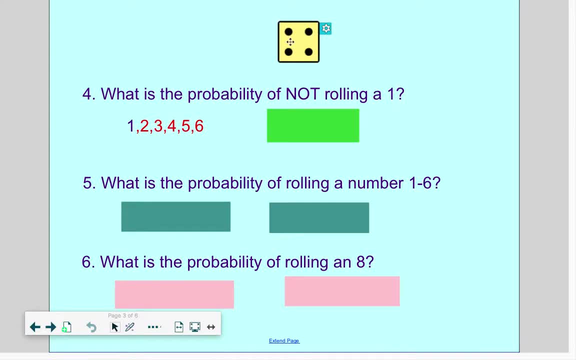 So I would say if we were rolling this die right here and trying not to land on a one, we have a pretty good chance of that happening. So I would say that is It's likely. Five, six means my probability is likely. 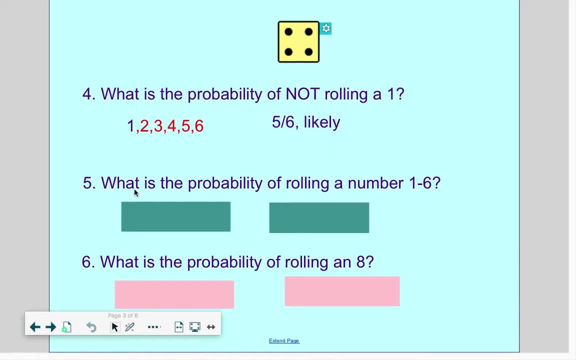 What's the probability of rolling a number one through six? Well, all of my numbers are one through six: One, two, three, four, five, six, Six out of the six numbers, six, six are one through six. 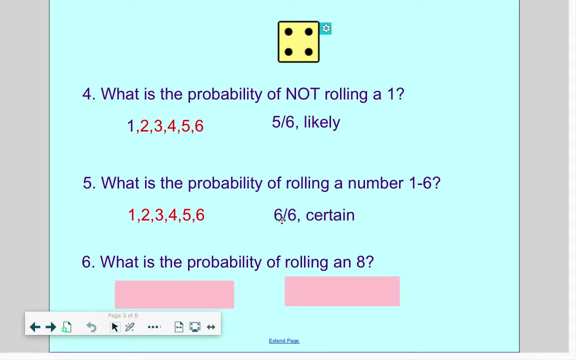 So, therefore, it is certain that I would land on a number one through six. What is the probability of rolling an eight? Well, I don't care how many times you roll this die or number cube, you can't land on an eight because there is no eight. 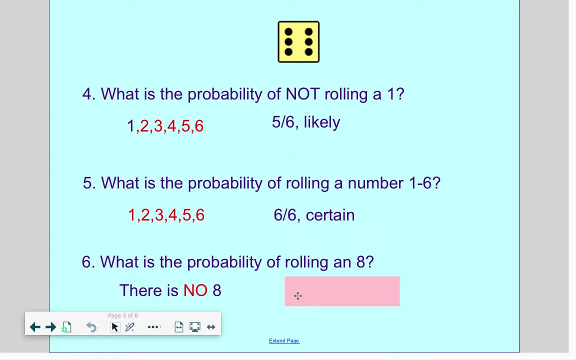 My numbers are one, two, three, four, five and six. So zero eights out of six, Zero six, which means none. Any time you have None of what they're asking about, it is impossible for it to happen. 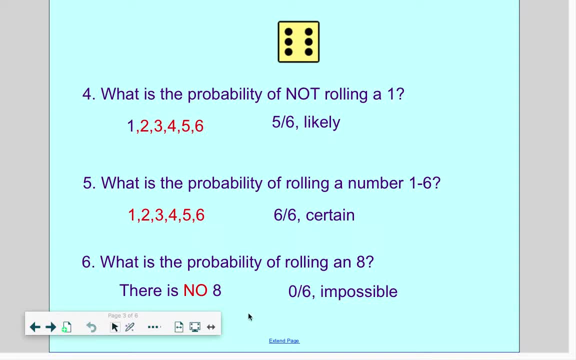 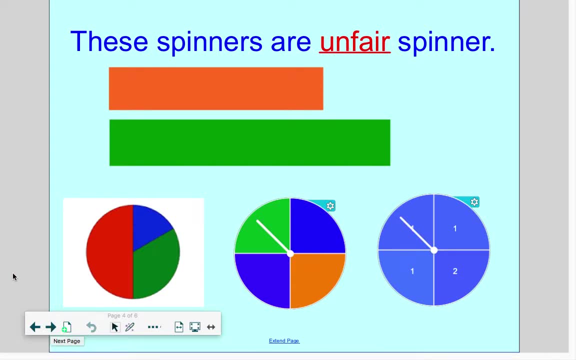 Now let's switch over and let's look at some spinners real quick. All right Below what you're seeing, these spinners are what we call unfair spinners. There are a couple things that make these spinners unfair. First of all, if you look at the spinner in front, 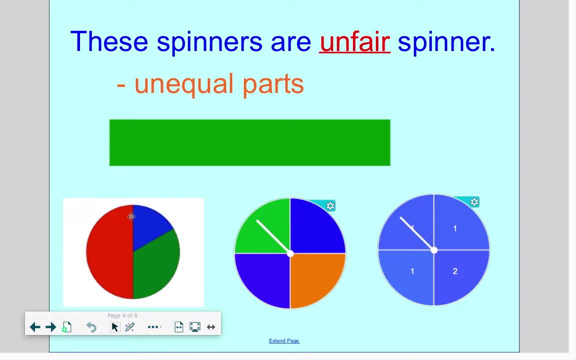 this spinner. This spinner right here is unfair because it has unequal parts. What color would you most likely land on here? If you said you would most likely land on red, you're right, because look at this huge section of red. Which color are you least likely to land on? 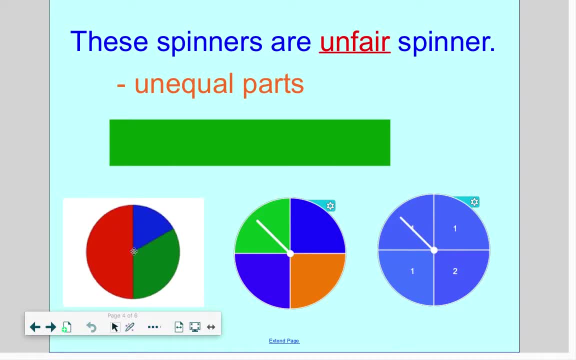 If you said blue, you're correct, because look at that teeny, tiny little piece of blue. Okay, So this spinner if we were playing a game? that isn't a fair spinner to use for a game because our parts are unequal. 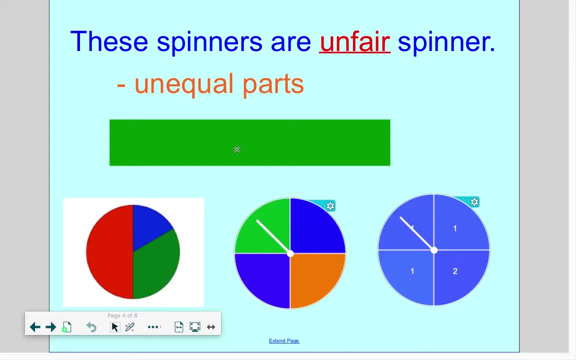 All right. When you look at the second spinner and the third spinner, these spinners are not fair spinners or unfair spinners, because the colors and their labels repeat. If you take a look at the second spinner, you have two blue sections. 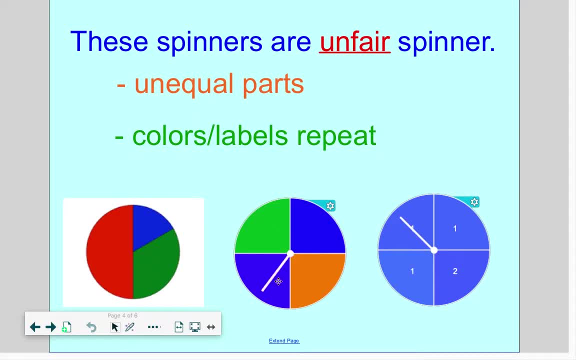 So we have a better chance of landing on the blue If we're spinning. See there, When you look at this third spinner. however, we have a one a one a one. We have a one a one a one. 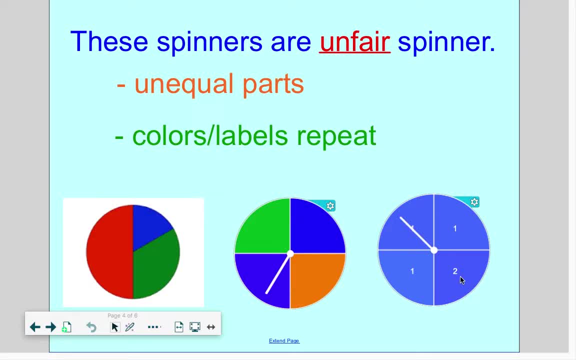 And then a poor little three all by- Excuse me- Poor little two, all by himself. So we have three ones and only one little bitty two. So which number are we more than likely to land on? We're more than likely to land on a one. 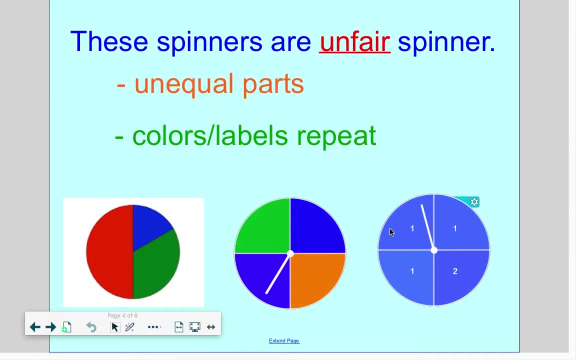 So that's why the third spinner is not a fair spinner. All right, Let's look at spinners that are fair And just Before I get off this page here, I want to talk about outcomes. Outcomes are the number of possibilities that could happen. 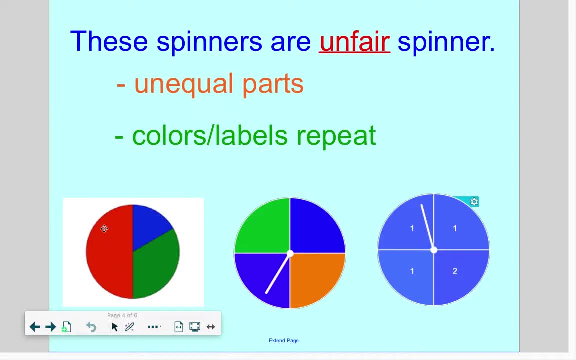 So if you're looking at this first spinner here, there are three outcomes for this spinner. We could land on a red, a blue or a green. So the first spinner has three outcomes. How many outcomes do you think on the second spinner? 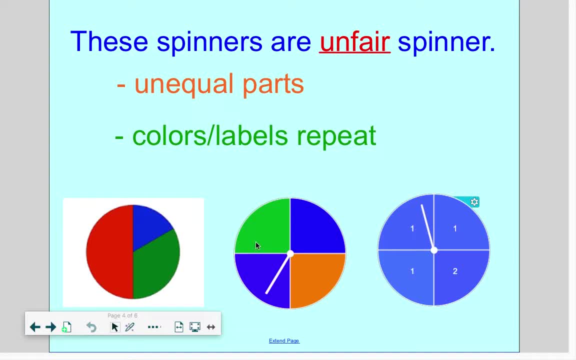 If you said three outcomes, you're right, Because we have a green, an orange or we could land on blue. So, even though this spinner has four sections, there's only three colors. Therefore, it's an outcome of three. 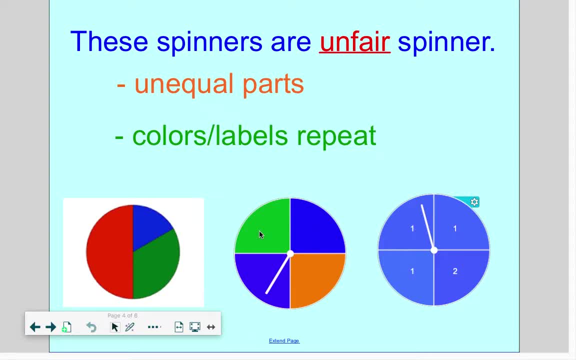 There's three different things that could happen. You could land on blue, green or orange. How many outcomes for the third spinner? How many different numbers can you land on? Well, you can either land on a one or a two. 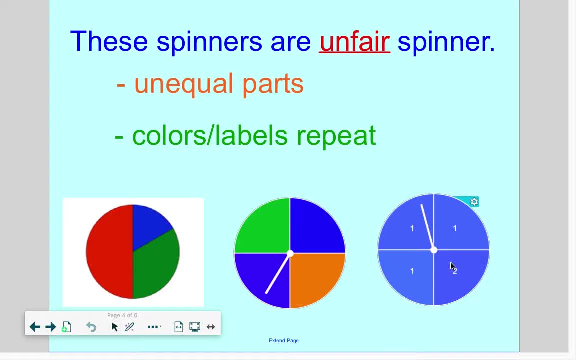 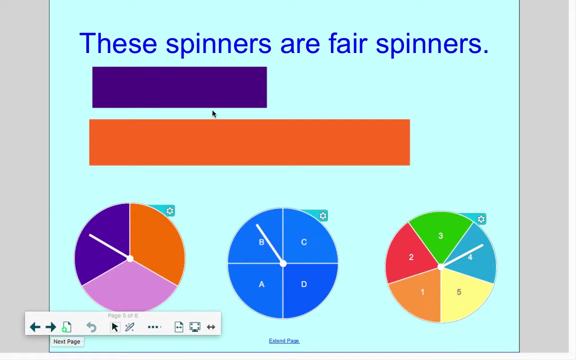 So my outcomes for the last spinner is two, Two outcomes. You can either land on a one or a two. Now let's take a look at fair spinners. These spinners that you see here are all what we call fair spinners. 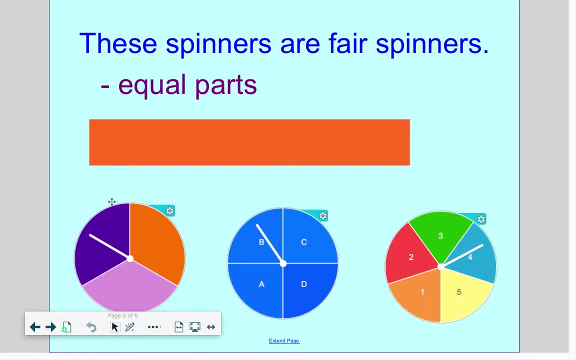 The reason why they're fair is they have equal parts. All these sections are exactly the same. They're all the same size. They are all equivalent pieces. Secondly, no colors or labels. repeat. If we're spinning the spinner right here we have a purple, a pink or an orange that we would land on.